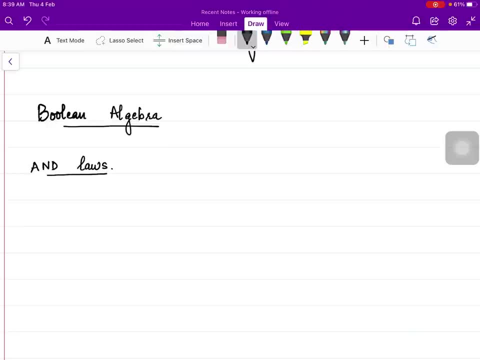 of AND gate is the product of AND gate. SO IN THE OF ist quote: AND gate is the product of AND gate. So the input of AND gate is the product of AND gate. SO you have to remember that if you have to know the input of AND gate, it is the result of a motor. If you 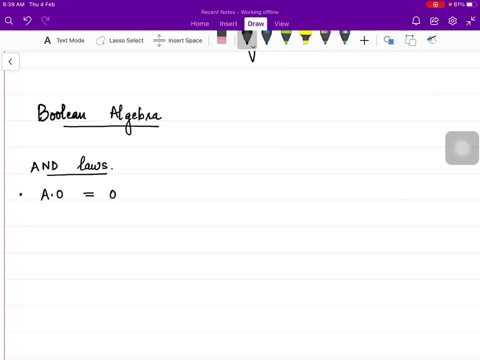 know how many motors there are in an enduring game? how many� artial dato are there in a coherent set of tuning? y yang nand n jing? you can type that in or instead of IN and PRONGING that IN as in PRO-PHASTIC, while we are studying both the inputs. So in this: 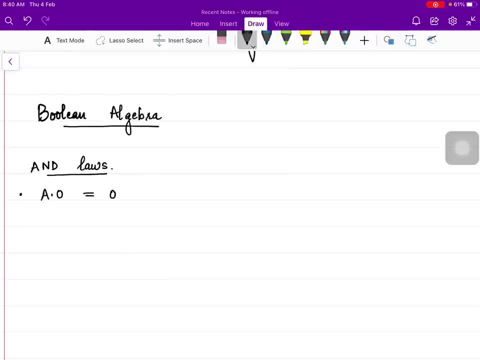 category. we will learn all the formulas that are related with the product. have to specially remember it. you already know it. then a.1 is equal to a. this can be also easily remembered because this is what we follow in normal maths also. then 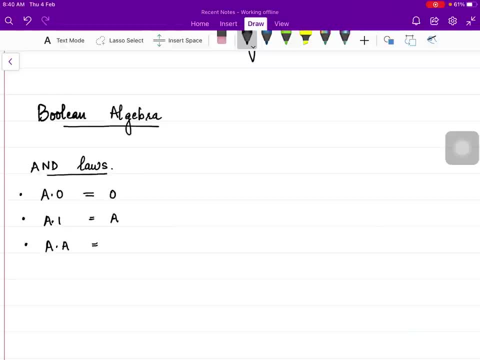 aa is equal to a, because a can be either 1 or it can be 0, so 1 into 1 is 1 and 0 into 0 is also 0, so when a is multiplied with a or you can say, aa will give you a in Boolean. 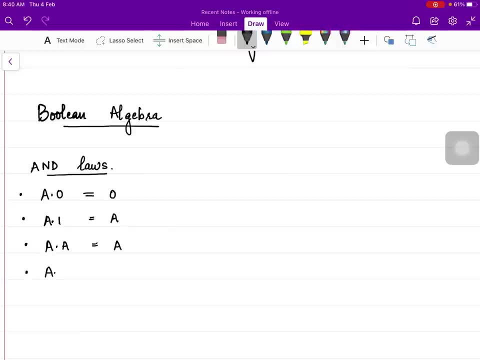 algebra aa, bar a can be either 0 or 1, so if a is 1,, a bar will be 0, because a bar is the complement of a. so if a is 1,, then a bar will be 0, 1 into 0 is 0, and if a is. 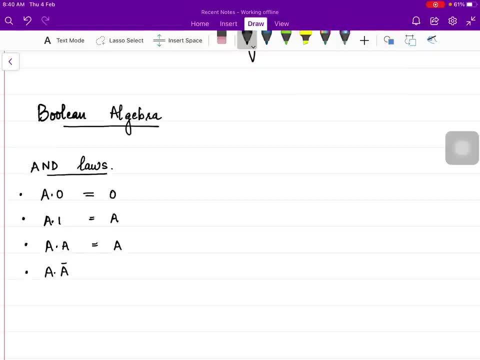 0, then a bar will be 1,, so 0 into a. So in any case it will give you 0,, so aa bar is 0,. so this was the first category of AND laws. Now we will study OR laws, as you all know that the output of OR gate is the sum of the. 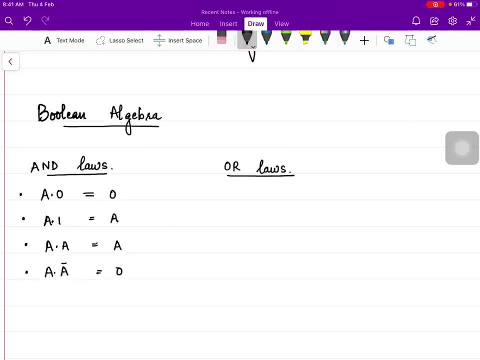 two inputs. so under this category we will learn all the formulas that is related to sum, Corresponding to the AND laws. we will convert the product sign into the sum sign. so a plus 0 will give you a, not to be specially remembered, we all know it. a plus 1, now everybody pay attention, a plus 1, see a can be. 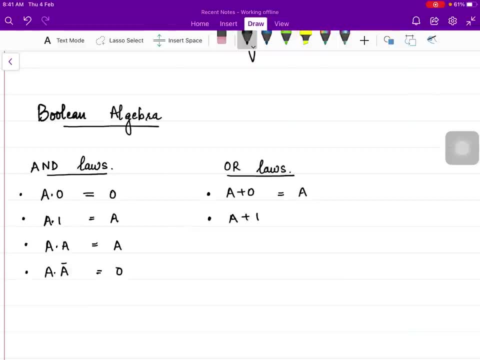 either 0 or it can be 1. so 1 plus 1 will also give you 1, and if a is 0, then 0 plus 1 will also give you 1. so if any of the inputs is added with 1, then you will get 1. then a plus a will give you a. 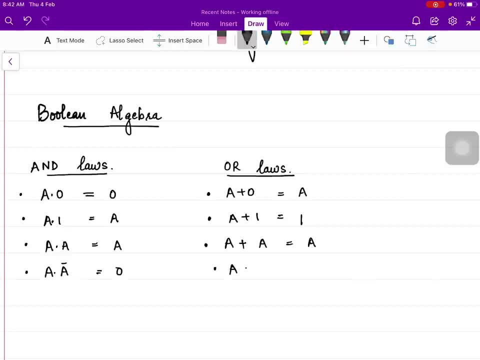 and a plus a bar will give you 1, not 0, because see, if a is 1, then a bar is 0, so 1 plus 0 is 1. and if a is 0, then a bar will be 1, so 0 plus 1 will also give you 1. 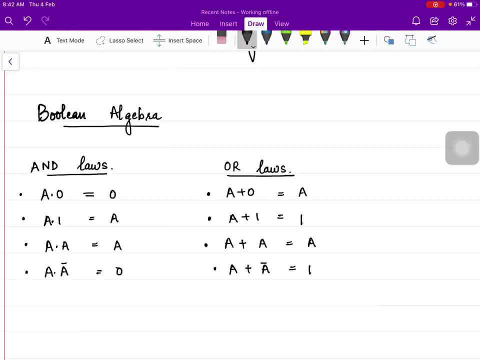 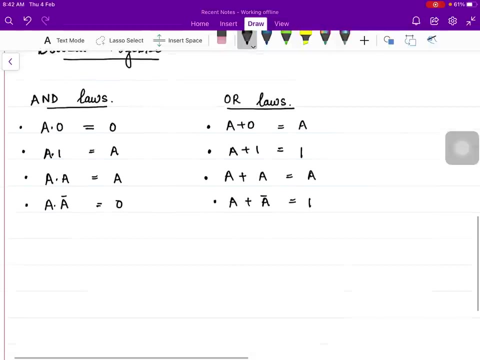 similarly, a plus 1 will give you 1. similarly, a plus a, if a is 1, then 1 plus 1 will give you 1. or if a is 0, then 0 plus 0 will also give you 0. so whatever will be the value of a, that will be the answer. so a plus a is a. so these are the two. 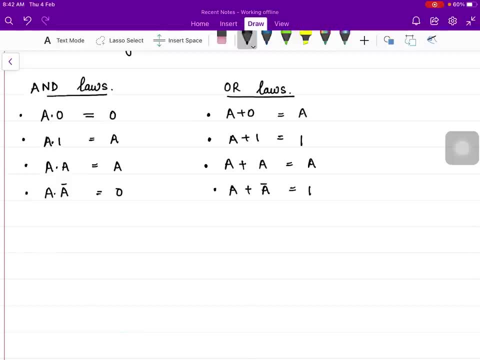 laws that you have to keep in mind. in total, there are four formulas that you have to keep in mind. so first category is add laws. second category is all laws. the third category is going to be the third formula. you can say it is the de morgan theorem. de morgan theorem. 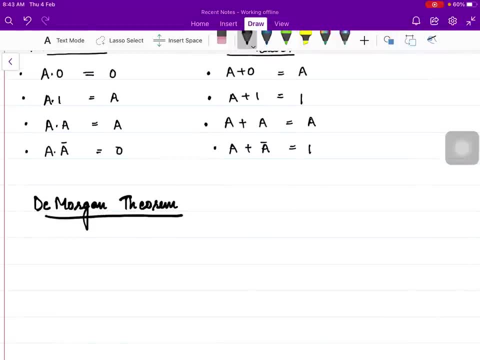 so what is de morgan theorem very, very important. see if a plus b whole bar. if you come across like this expression, so the answer is a bar, you will individually put bar on both the inputs, but the sum sign will become input of the inputs. so the answer is a plus b whole bar. if you come across like this expression, 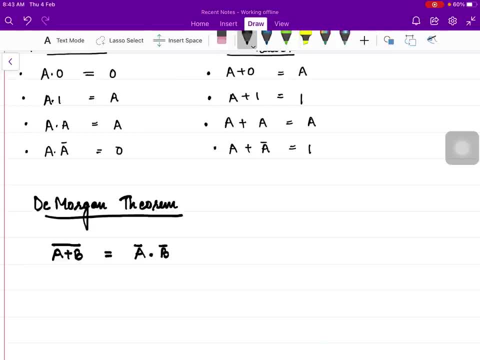 into the product sign that is a bar, dot b bar. similarly, if you have a dot b whole bar, then you can break it as a bar b bar, but the product sign will get converted into the plus sign. so it is a bar plus b bar. this is de morgan theorem very, very important. so this was 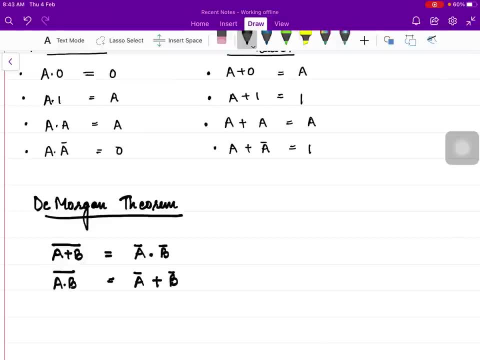 the third law that we have to keep in mind while solving the expression, and the last one is a simple formula. the formula says that if you find an expression like this, that is c plus a d, it can be simply written as c plus a into c plus d. this is the fourth law that you have to keep in mind. 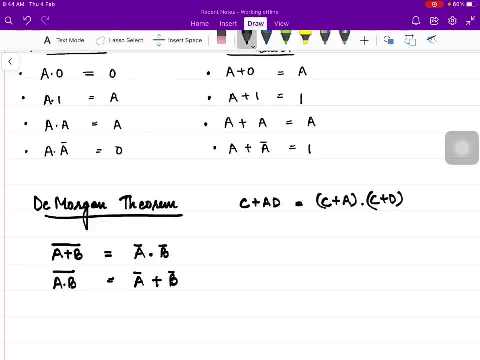 so these four categories you have to keep in your mind while solving the expression, and you will be easily able to solve or minimize any of the expressions by the use of these four laws. so just keep them in mind and you can solve any of the expressions. so c plus a, d will give you. 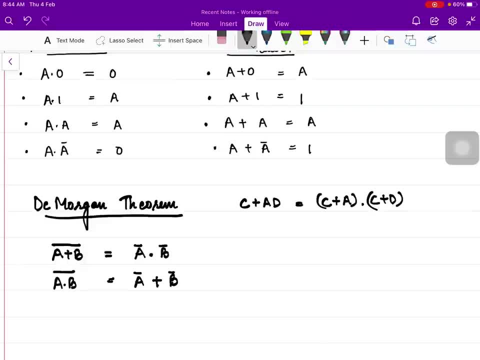 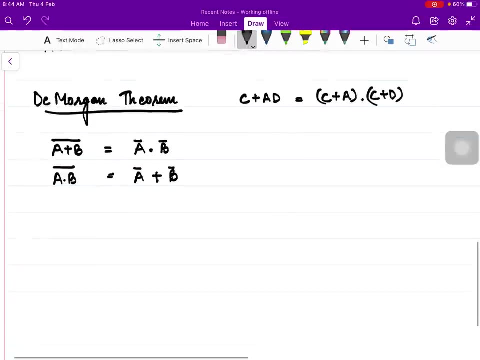 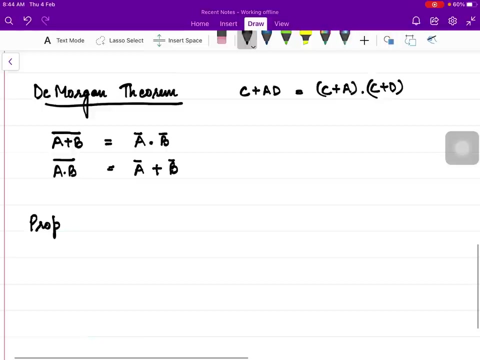 the last one that we have discussed, that is, c plus a- d. if you find come across any of such expressions, then it can be broken as c plus a into c plus d. okay, so now let us also read or discuss, the properties of the boolean algebra. properties of boolean algebra. 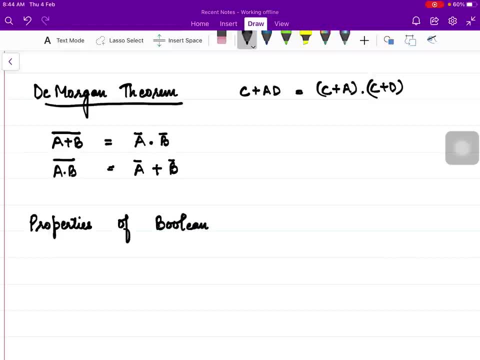 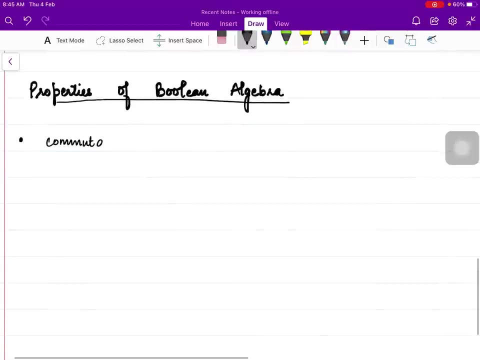 the first property is commutative law, commutative law. so see, what we have to do is we have to find the properties of the boolean algebra. what is? the commutative law says that a plus b is equal to b plus a. you follow this in maths. 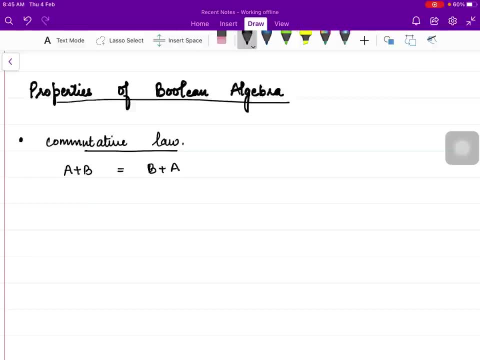 also. so there is no big thing. in your normal maths also, you will always follow it. we all know that a plus b is equal to b plus a, or a dot b is equal to b dot a. so this is commutative law. i hope it is understood by all now. the second one is associative law. associative law. 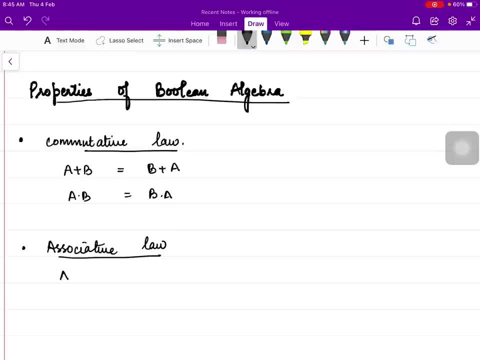 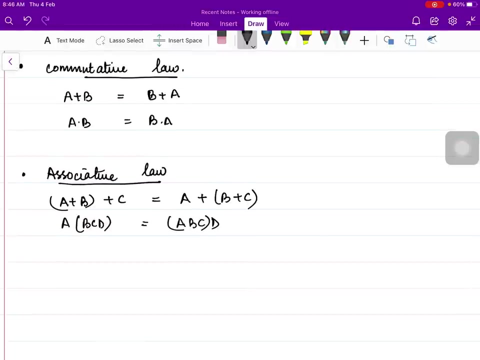 what does the associative law say? a plus b plus c is similar or is equal to that of a plus and b plus c. similarly, a bracket, b, c, d is same as that of a, b, c in bracket and d outside. this is same. so this is associative law. we all know it. but the main thing is that we don't know what type of property. 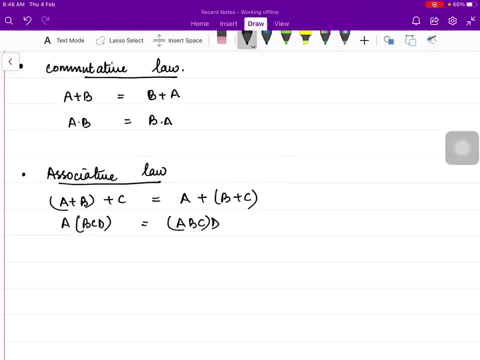 is this. so we all know that this is associative law. so we all know that this is associative law, we all follow it, but we don't know what is the name of the property. so we should remember what is commutative law, what is associative law and what is distributive law. the third and the last. 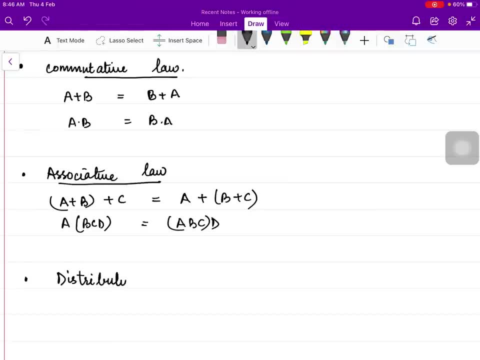 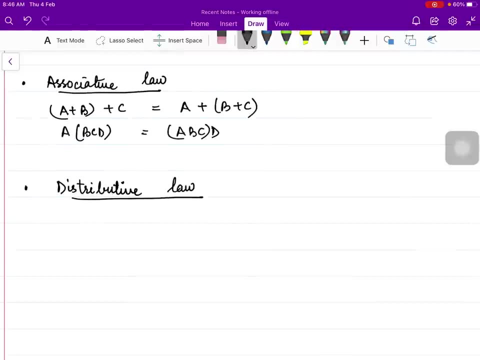 one that is distributive law, which are followed in the same manner here also as we follow in our normal maths. that is, a into b plus c can be written as a b plus a c. so this is distributive law. so all these are the properties that are followed by boolean algebra or which are valid. 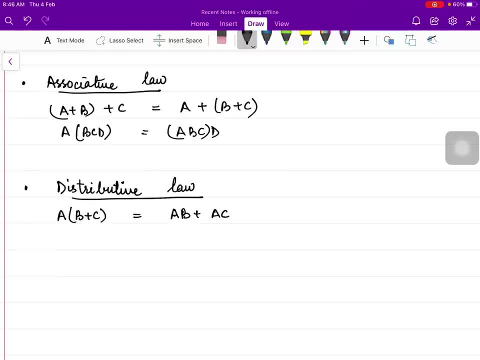 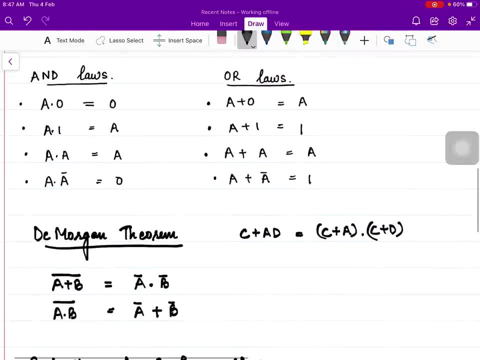 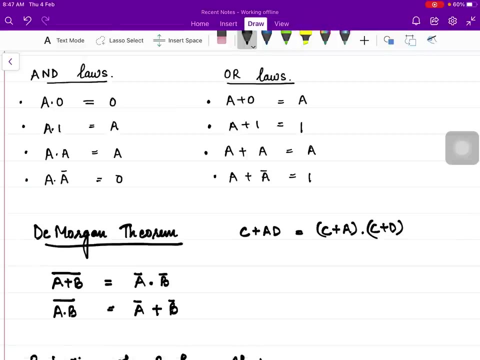 for boolean algebra and the four laws that we have to keep in mind while solving the boolean expressions. we have already discussed them. that is, and law or law, and de morgan theorem and the fourth formula, that is c plus a d. so these are the four main laws that we have to keep in mind. 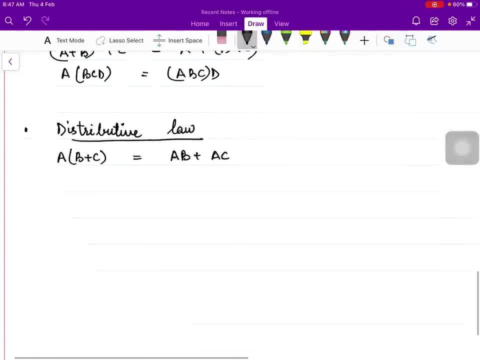 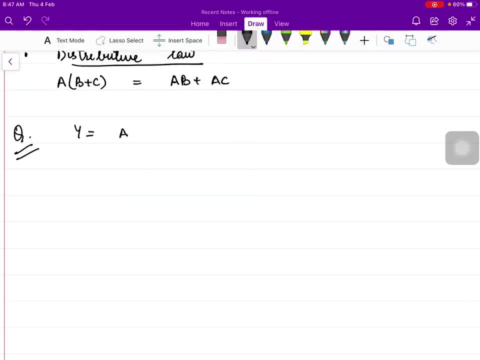 so let us start solving some of the boolean expressions, like first one is: y equals to a bar b plus a b, bar plus a b. we have to minimize this expression. so how will we minimize? you can solve. the method of solving can be different for different students as they visualize the question, but the answer will come. 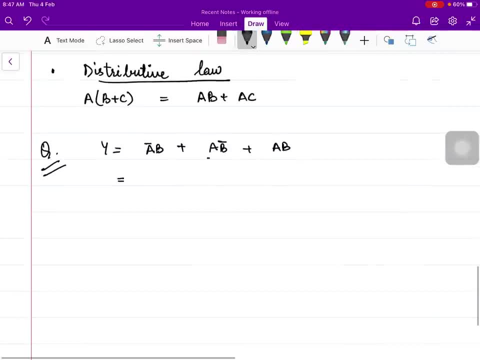 out to be same. so from here, from these two terms, we have to minimize this expression. and if you do the same thing again in terms of this equation, let me tell you what we should learn from this garden. in the two terms, I am taking a common, so we will be left with b bar. 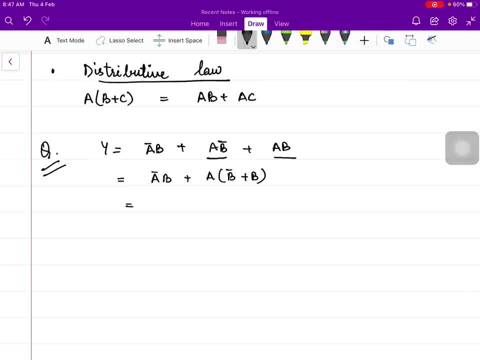 plus b and according to the law, or law b bar plus b will be one. so a bar b plus a, a dot one will be only a. now you can see plus ad, the formula that we discussed earlier. you can. according to that, you can break this like you can break the above expression like this: 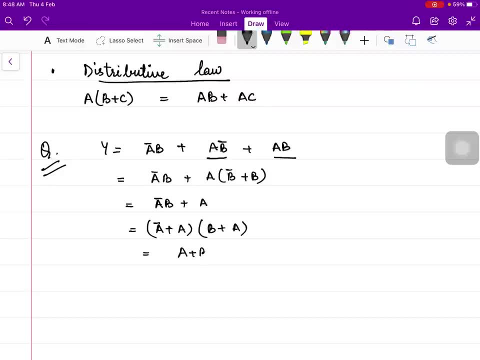 a bar plus a is equal to a nd. this expression- together both are their same, so let's start with a- will give you 1, and you are only left with a plus b. So the answer is a plus b. This is how we will. 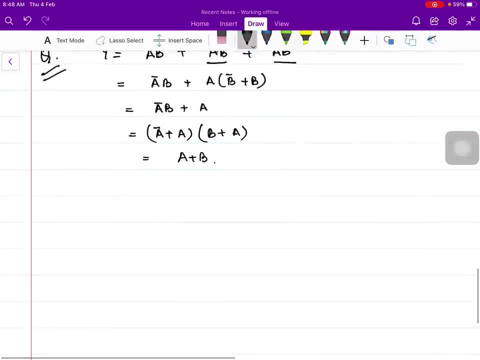 solve the expression. Similarly, if we move on to the second question, y equals to a bar b bar c plus a bar b c bar, plus a b bar c bar plus a b bar c. Okay, so how will you solve it? I am taking b bar c common from these two expressions which I have underlined these: 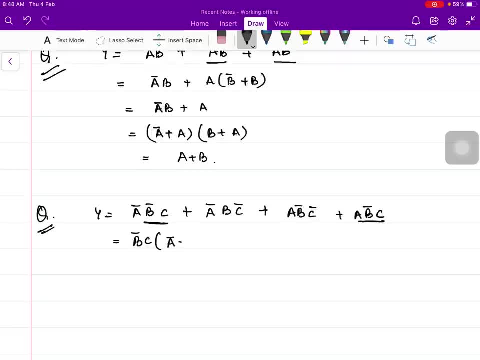 two terms. So b bar c, a bar plus a will be left in the bracket and it will be a bar b c bar plus a b bar c bar plus a b bar c bar. So this is how we will solve the expression. 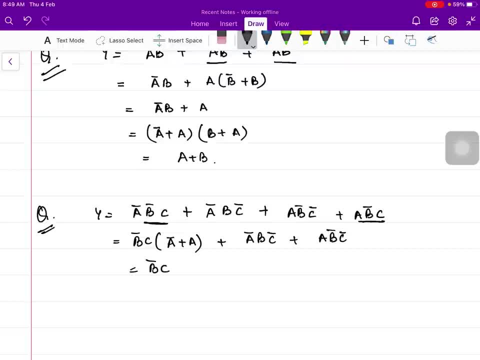 a b bar c bar. So it will be only b bar c plus a bar b c bar plus a b bar c bar. Now I think we can take b bar common from here, from here and here. So I am taking b bar common. 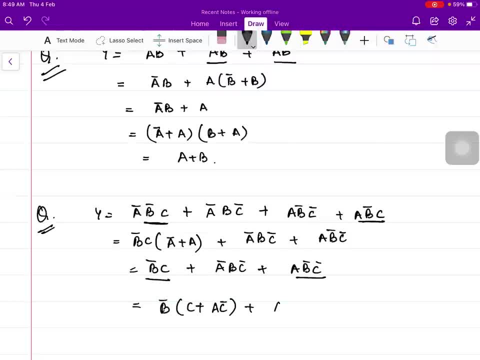 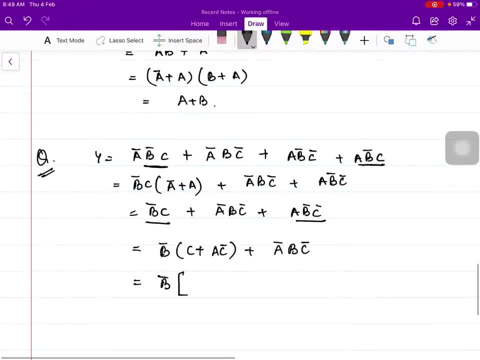 and c plus a, c bar plus a bar, b, c bar. Now the b bar and the- The terms which are in the bracket can be broken like C plus A, into C plus C bar plus A bar, B, C bar. So it will be B bar and you will be only left with C plus A, because C plus C bar will become. 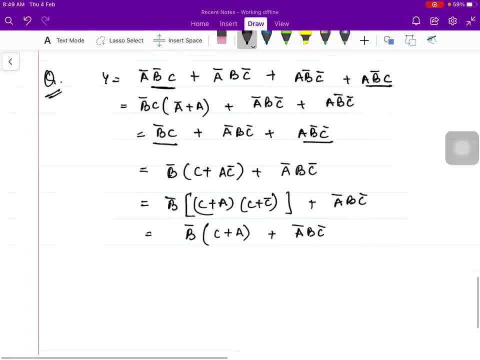 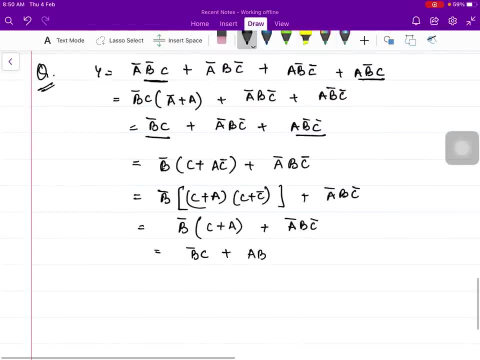 1 plus A bar, B, C bar. Now I don't think that further solution is possible. So we will open the brackets And we are left with this answer. So we can minimize the above expression maximum. till here Further solution, or you can say further minimization is not possible. 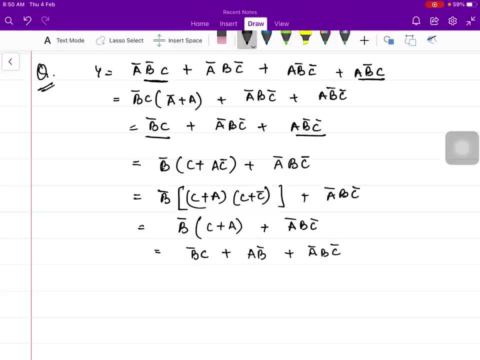 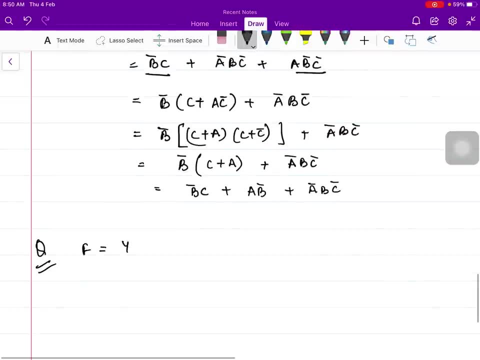 Okay, so this is how we solve the various Boolean expressions using Boolean algebra. Let us do one more in the last question. F equals to Y bar Z bar plus W bar, X bar Z bar plus W bar X bar. Y bar Z bar plus Y Z bar. 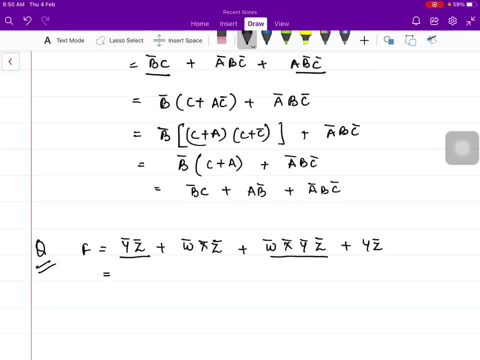 Now what you can take: Y bar Z bar. you can take common from here. So you will get 1 plus W bar X bar plus W bar X bar Z bar plus Y Z bar. So Y bar Z bar 1 plus any input is 1.. 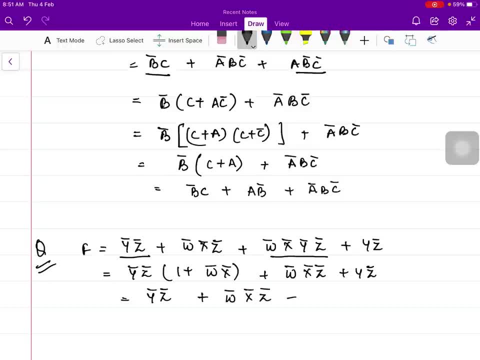 W bar X X bar, Z bar plus Y Z bar. Okay, so now you can take Y bar or you can take Z bar common from here, So you will be left with Z bar, Y bar plus Y plus W bar, X bar, Z bar. 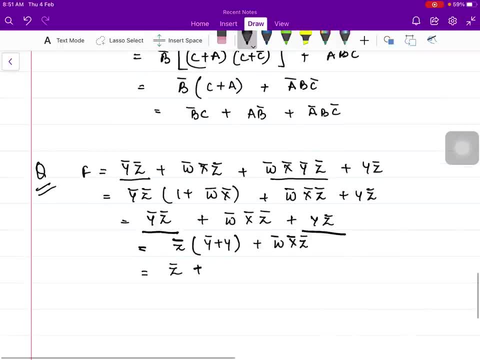 Now Z bar. only Z bar is left, because the this term becomes 1.. And W bar X bar Again. I am taking Z bar common 1 plus W bar X bar 1 plus any input is 1 and it is only Z bar. 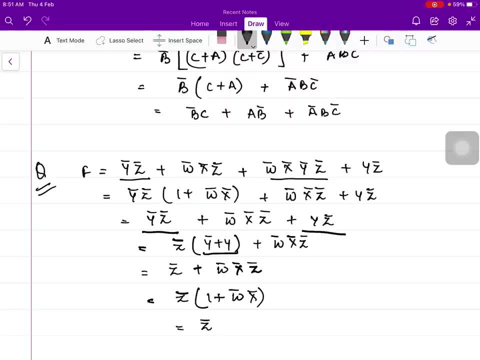 So this is how we solve various Boolean expressions using Boolean algebra. I hope it must be clear to all. One trick that I will like to tell you is that first of all you should copy the question correctly from your question paper into your algebra. 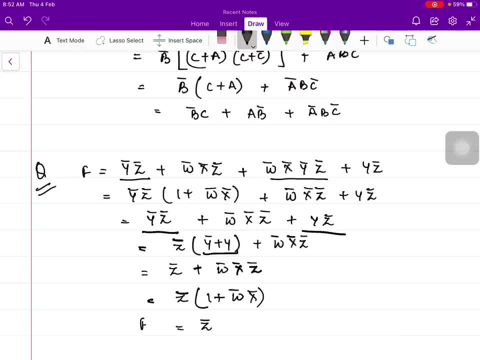 Because the expressions sometimes are so complicated that if you don't copy them correctly in your answer sheet, the mistake will begin from there itself. All right, so always doubly check when you will copy the question from your question paper to your answer sheet, when you will copy this expression to solve in your answer sheet. 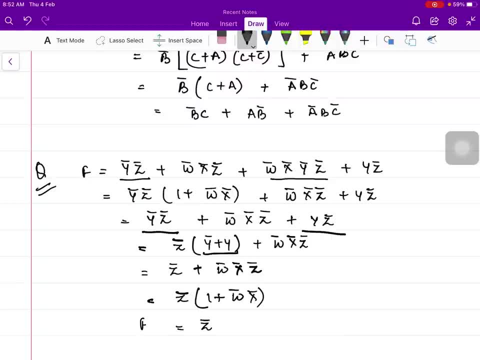 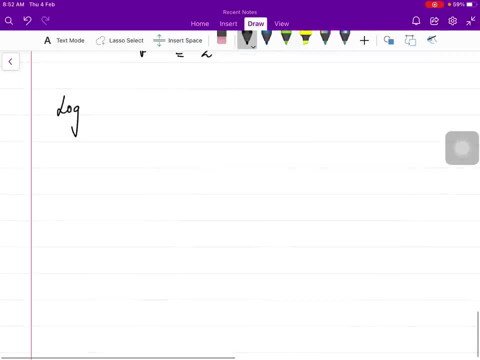 So doubly check it from the question paper. So this was the Boolean algebra. Now let us start discussing the logic Of which you, many of you must have already heard: logic gates. So basically there are three basic gates, And what are they? and gate, or gate and not gate. 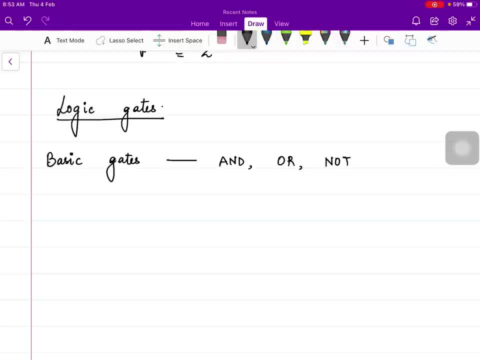 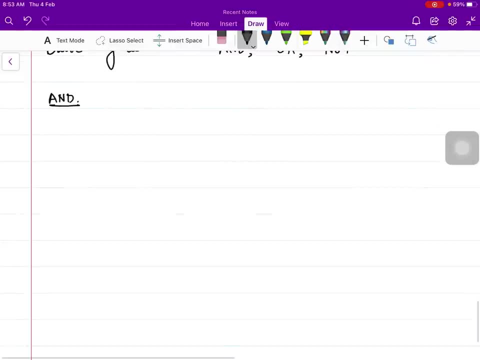 These are the three basic gates. All right, So first of all, let us discuss them. And gate In laboratories. you will get the IC for each gate, but the way you represent them is like this: This is how we represent an AND gate. 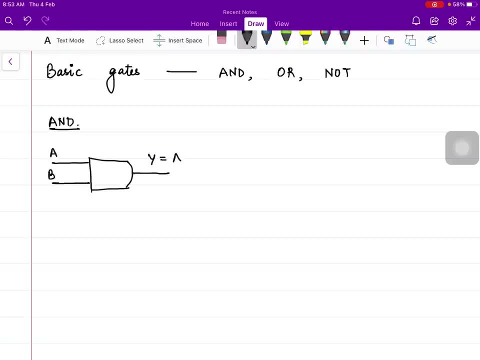 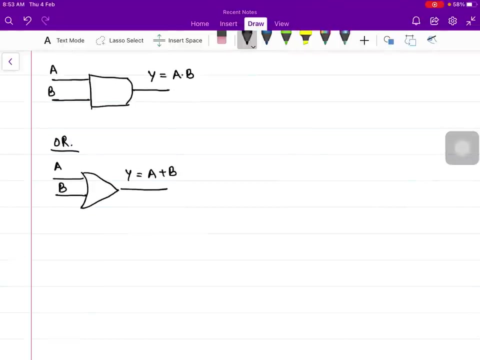 These are the two inputs, A and B. Output is Y and Y is A dot, B, Okay, OR gate, Two inputs. Way to represent is like this: OR gate And the output is Y, which is A plus B. OR gate gives you the addition of the input and AND gate gives you the product of the inputs. 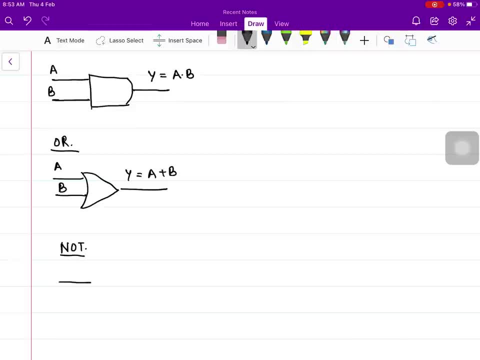 Now not gate. not gate is also called inverter single input Bubble. having a bubble- This bubble has a very- is very much significant. It has a great significance. wherever you will find this bubble, That means the input will be inverted. at the output that means you will get a bar. so if a is 0, it will. 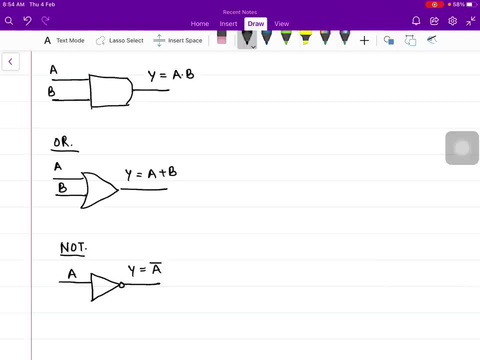 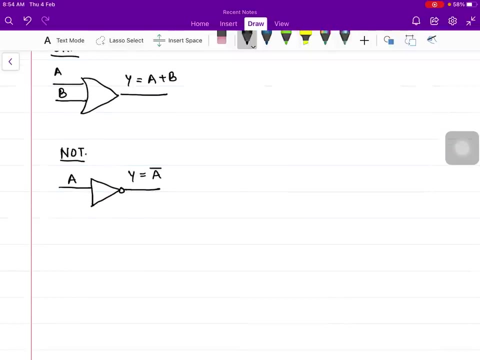 become 1, and if a is 1 it will become 0. so not gate is also called inverter. so these are the three basic gates, logic gates, that is, and or and not now universal gates. we have one more gate, which we must all know, that is, but that doesn't come under the category of basic gates, that is. 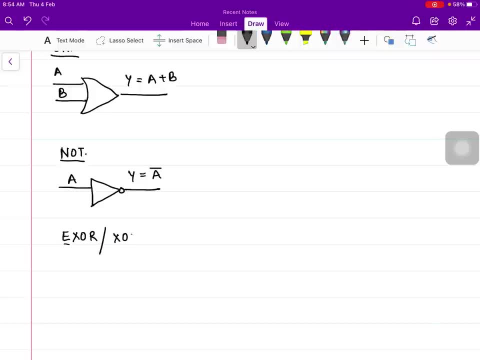 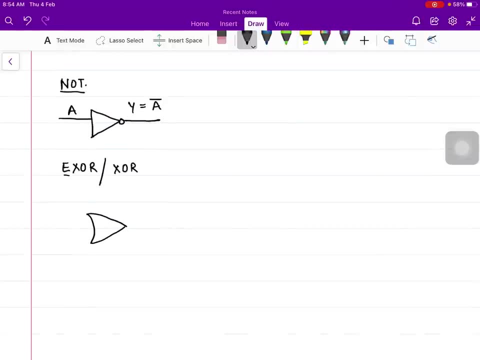 exorgate. all right, we also write it like this. we also write it like this: now, what is exorgate? as it includes the name or, so it will certainly have the symbol of or, but an extra line like this: this is how we represent an exorgate: y is the output and the expression of output is: 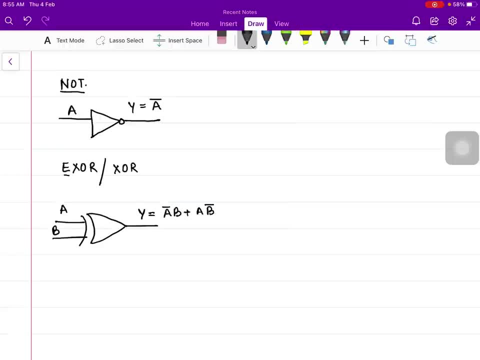 a bar b plus a b bar. we have to remember it: a bar b plus a b bar. and the sign of exorgate is like this. so this is the symbol of exorgate. this is the expression of exorgate. y equals to a bar b plus. 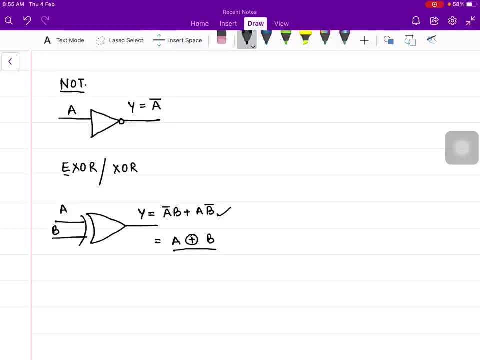 a- b bar, and it can be also represented like this when you will make the truth table of exorgate. so the combination can be 0 0 0, 1 1 0 and 1: 1. the technique that you have to remember, either you put, 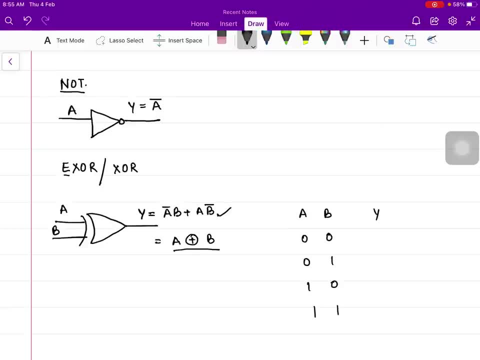 both the values of a and b in this expression. or you can simply remember like this that if both the inputs are same, that is 0, 0 and 1, 1, so the answer you will get is always 0. you can verify them by putting into this expression: and if the inputs are different, you will get an output of 1. 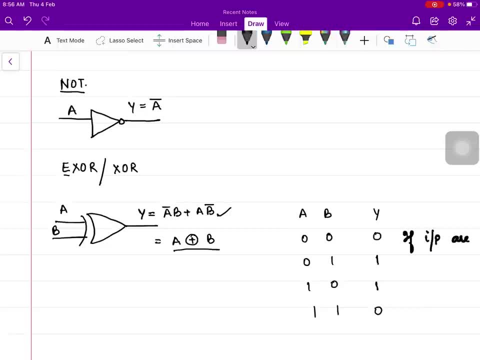 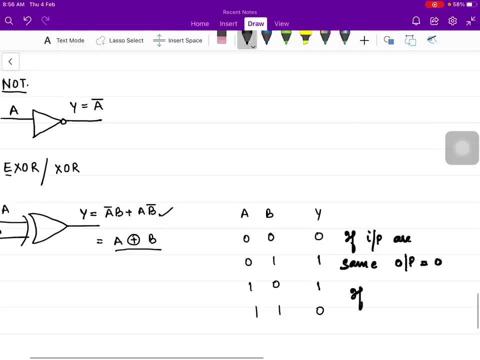 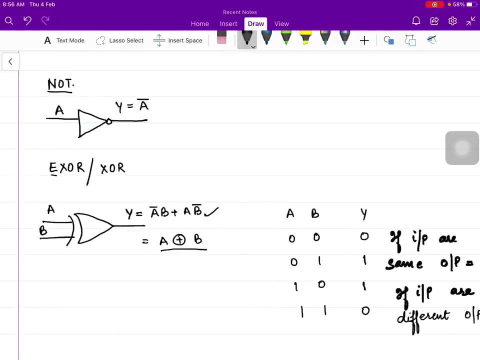 so if inputs are same, output is equal to 0. if input are different- one is 0 and other is 1- then output is always equal to 1. so this is how the exorgate work. similarly, we have an opposite of exorgate, that is x'th'. 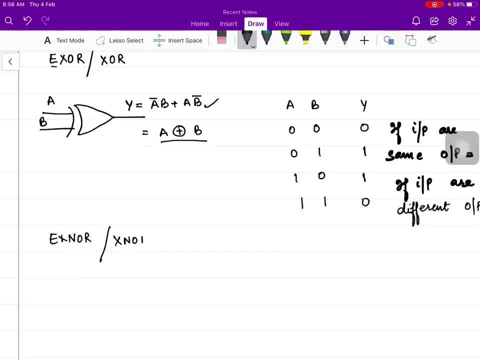 gate. it's also written like this: how do we represent it? first of all, make an XOR gate and I have told you the significance of bubble, so it will just invert the expression. so when you will invert the whole expression, you will get a bar, b bar plus a b, a Barbie bar plus a- b, and you can also represent it like: 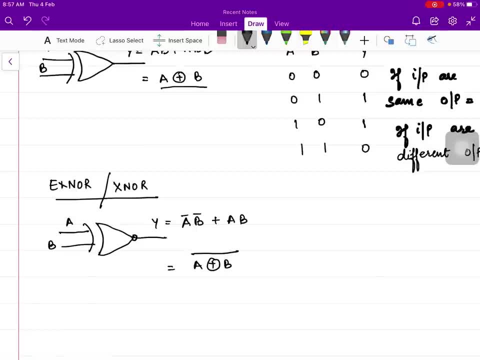 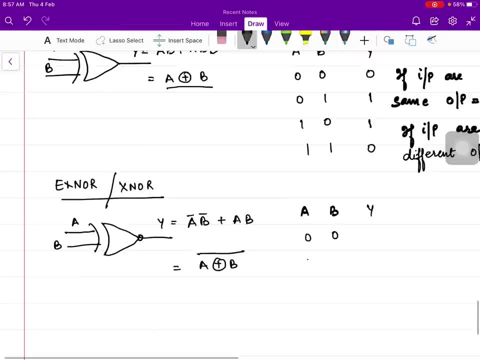 this. first of all, you will write the expression of XOR gate. take the total bar, alright. and while making the table, you have to remember the concept opposite to that of absorb, that if both the inputs are same you will get an output one, and if both the inputs are different, you will get an output 0.. You can verify it by putting. 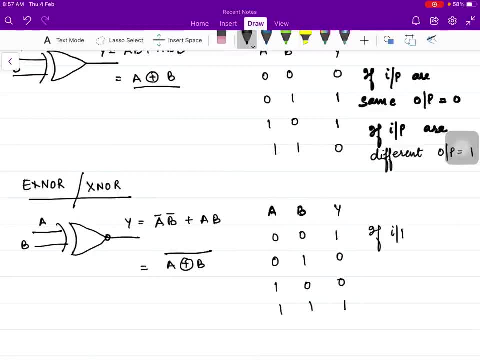 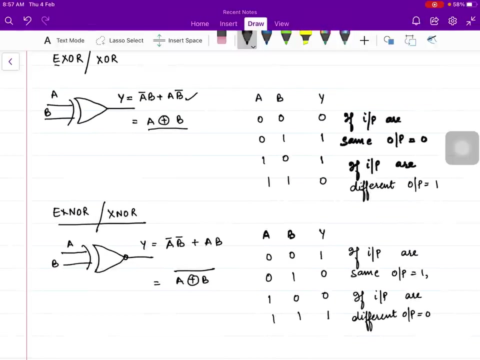 into this expression: If inputs are same, output is 1.. If inputs are different, output is 0.. So I have told you that X0 gate is the opposite, or you can say the complement of XOR gate. So what was XOR gate? a bar b plus a b bar. Alright, So how does this? 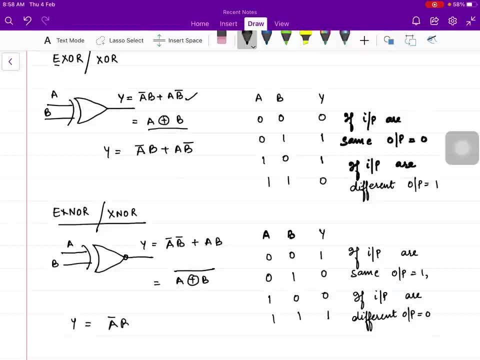 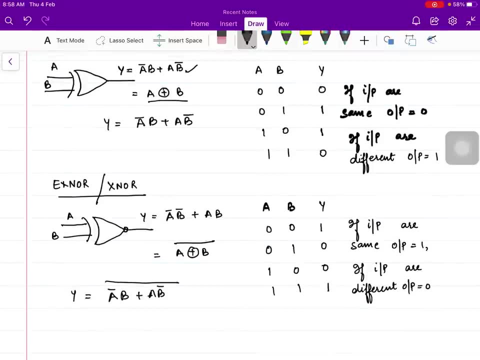 come a bar, b bar plus a, b. See, you have to take the total bar of the expression. like this: This was the XOR gate and when we complement it, that means we have to take the whole bar and then you will solve it by De Morgan theorem. When you will solve? 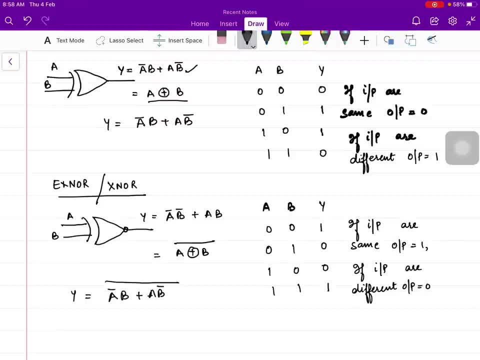 it, you will find out that the expression comes out to be a bar b bar plus a b. So do not get confused that ma'am is saying that the X0 gate will be the complement of the XOR gate. Then why have not we written the complement? Why have we written a different? 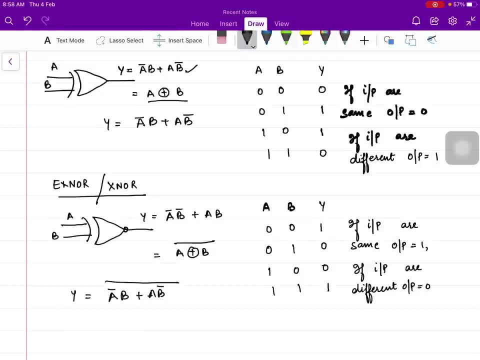 expression: a bar b, bar plus a, b. So that is the same. That is, we have taken the complement of XOR gate, and when you will solve it by the complement of the XOR gate, then you will solve this expression five times. Now we have half the axioms and half the slipped. 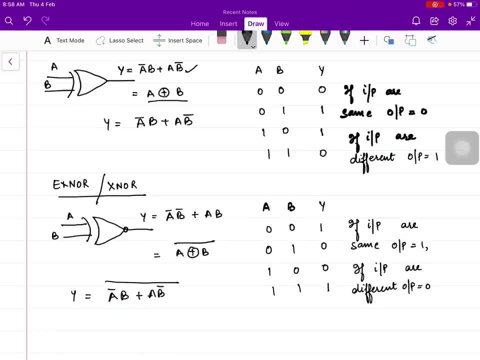 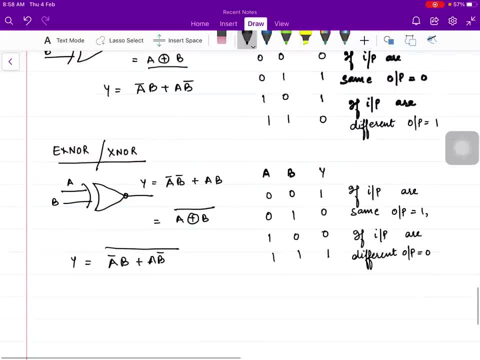 answer. Now we have a function forY 2 which is like this: x is mu plus w times 1.. Now in this case we are saying x plus 1. That will be like a 10 times. So it means that if we� 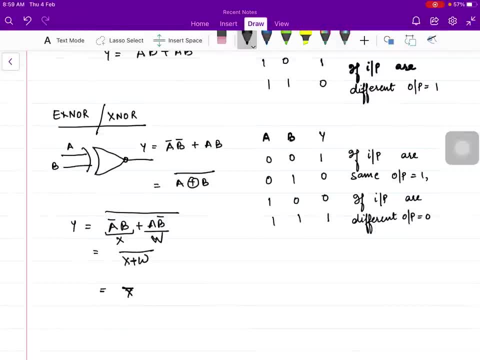 right say of jakimorgon theorem. now it is like It is like you are saying that x to case is equal to w. That is the expression for Engineering vars of the domain. Well, we have seen that this was gradient. you have come to this expression. 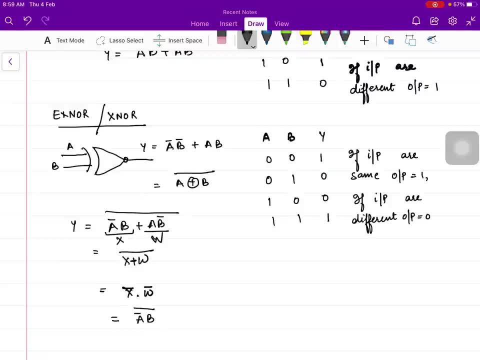 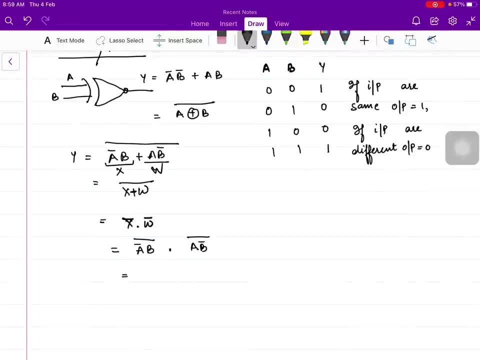 blue bar. so what is x a bar, b whole bar. dot a b bar, whole bar. Now further solve it by De Morgan theorem. this part, that is a bar bar plus b bar, The product sign will get converted into plus sign by De Morgan theorem. dot a bar plus b bar bar. So a bar, a double. 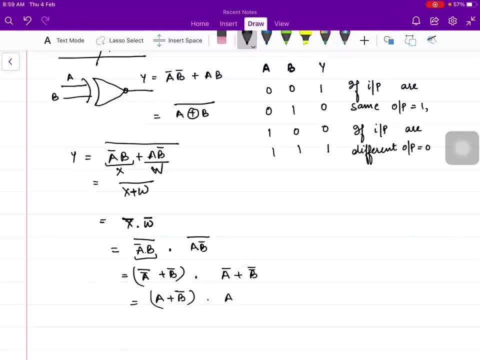 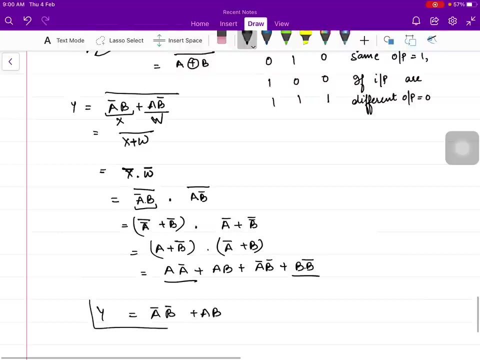 bar gives you a plus b bar. dot a bar plus b. If you open this bracket, you will get a, a bar plus a b plus a bar, b bar plus b. dot b bar. This term and this term will be 0.. So what is left with a bar b bar plus a b. That is what is the expression of x naught. 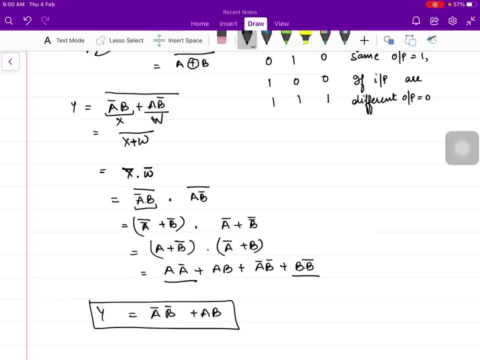 gate. Alright, so these were the givens. Now let us come back to the basic gates. The basic gates were three, that was, and, or and not. but we must also know the expression of xor and x nor gate, because they will be helpful for us in highest when we will move forward in digital electronics. and now let us come. 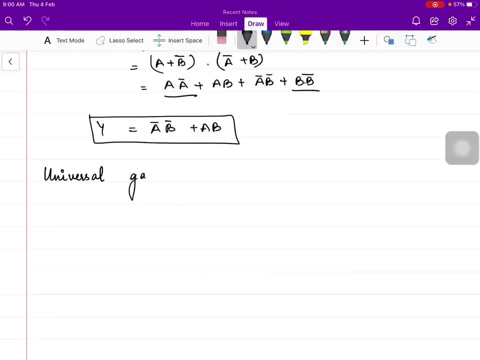 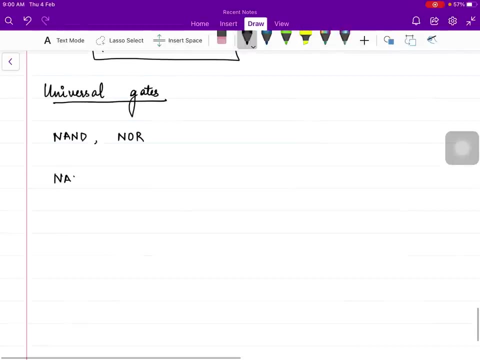 to the universal gates. So what are the universal gates? We have two universal gates, That is, and NOR gate. okay, so first of all, let us see what is NAND gate. how do we represent it? first of all draw an AND gate and then a bubble. so what is the? 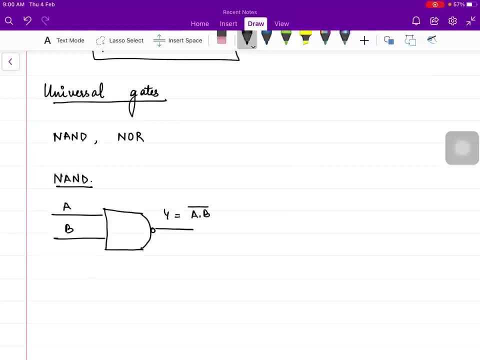 expression, you will get a dot B whole bar. similarly, what is NOR gate? draw an OR gate. first of all, bubble becomes a NOR gate. AB are the inputs and Y equals to A plus B whole bar. it is the NOR gate. now the question arises that why are 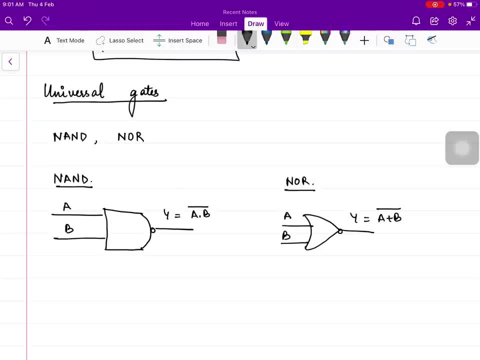 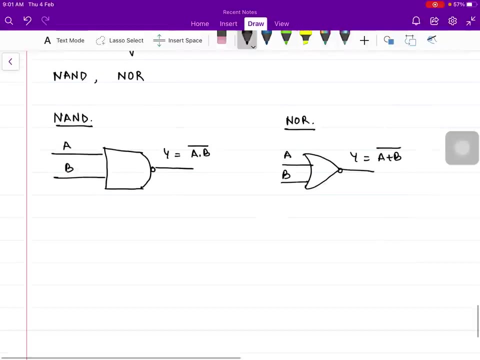 they called universal gates. they are called universal gates because by using only NAND gate or by using only NOR gate, you can realize any of the gates. okay, let us see how AND gate. first of all, I will construct all the gates using NAND gate. okay, so first of all, let us do AND gate, let us realize AND gate by NAND gate. 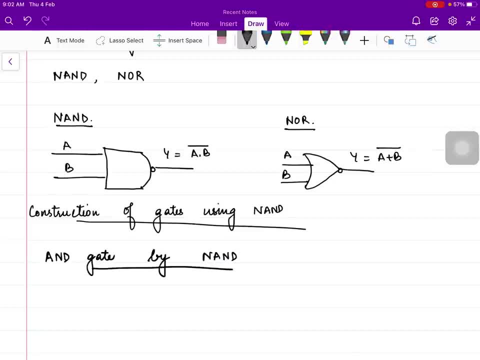 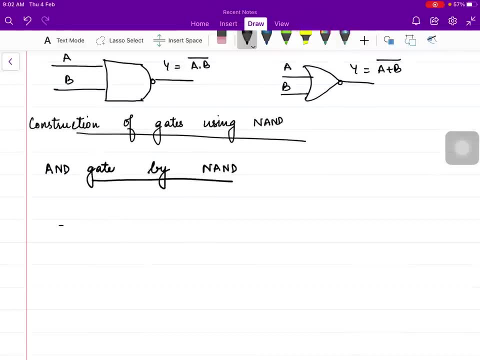 see what is the expression OF: AND gate that you should get at the output a dot be and you have to use NAND gate only. so NAND gate is like this: A B, okay, so you will get here a dot B whole bar, but you wanted only a dot B, so put another NAND. 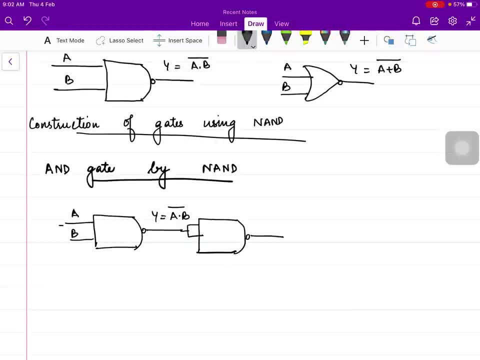 gate shortly to inputs, because you have to give only one input. that is the output of this first nand gate and you will be getting. let the output be z a dot b, because it will be. it will take the bar of the y, so it will be a dot b. 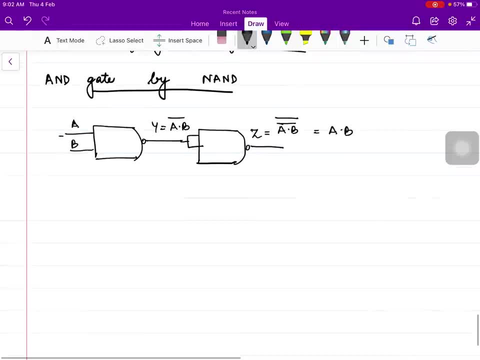 so and gate is made by using nand gate. similarly, if we talk about or gate by nand gate. so what is the output of or gate that we want? we want a plus b, and nand gate gives you a dot, b, whole bar. so what we have to do, we have to take two nand gates. 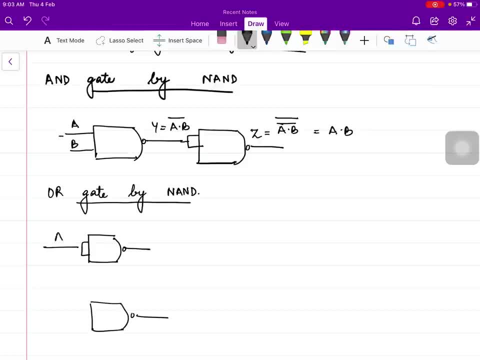 short the two inputs and put one here. a short the two inputs, b, that's a. okay, so here you will get a bar and b bar. now put the third gate here, nand gate. what you will get here a bar dot b bar, whole bar. apply the de morgan theorem. 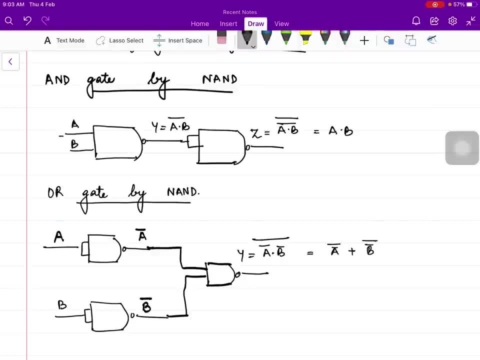 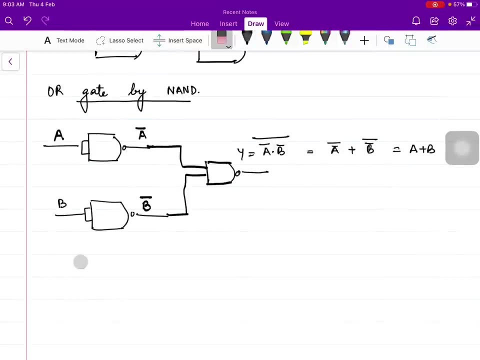 a bar bar plus b bar bar, that is a plus b, so it has become the or gate. you can realize the or gate also by using only and only nand gate. now, not gate, not gate. very, very simple to realize the not gate by using nand gate. so you will get a bar, dot b bar, whole bar, dot b bar, whole bar. apply the. 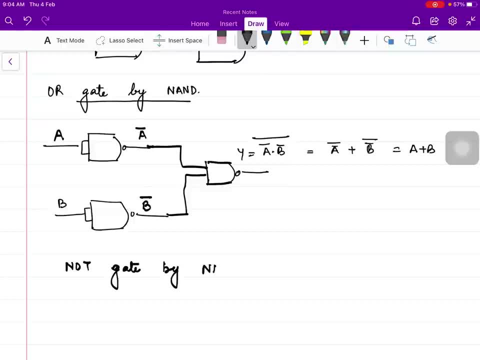 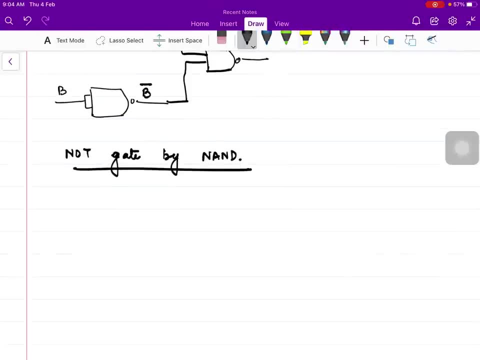 nand gate. what is the output of not gate? that is a bar and nand gate gives you a dot b whole bar. so put the, put a single nand gate short. the two inputs we have to feed only one input. sorry, i am writing a bar again and again. it is a and you will get a bar here. so it is a, not gate. 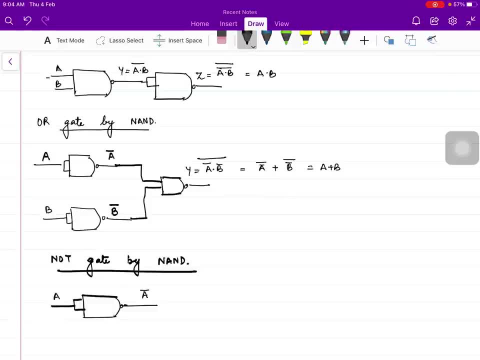 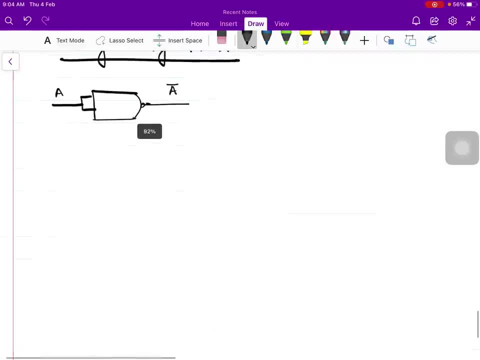 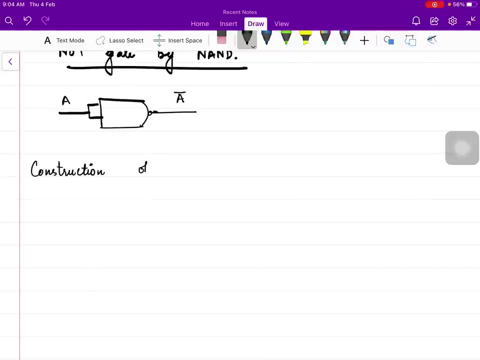 so this is how, by only using nand gate, you can realize all the gates. so that is why nand gate is a universal gate. similarly, we can realize all the gates by using not gate. first of all, let us realize and gate by nor gate. so what is the output of? and gate? a dot b that we should get, and the output of not gate is a plus b. 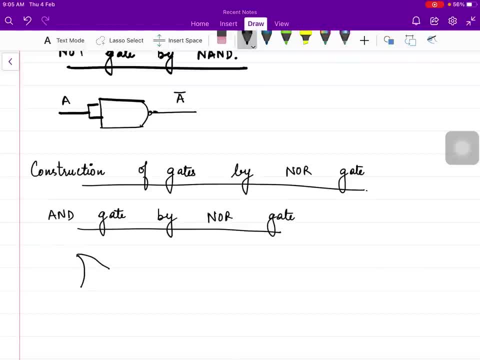 whole bar. so we will put a nor gate, short the two inputs: a, we will get a bar here again, a nor gate. b, we will get b bar here, and if you put another nard gate here you will get a bar plus b bar, whole bar. so what is the de morgan theorem? A bar bar, dot b bar bar, it will give you a dot b. so this is the and gate. 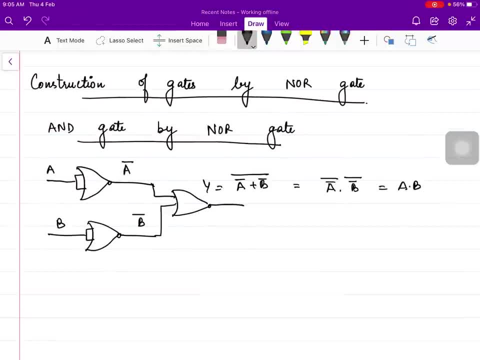 by using, not gate. so whenever you have to, you can remember it like this: whenever you have to Realize a and gate this, this means that I can add a nothing or no now www money or allows to find the bar a just on my side for the network. 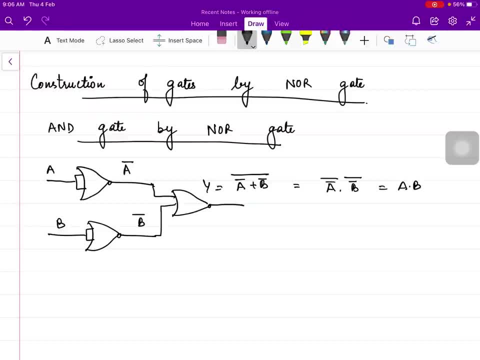 end realize OR gate by NAND gate. then you have to put the three NAND gates in this manner, that is, three NAND gates and you have to feed. you have to short the two inputs of the two NAND gates and feed one, one input to that. then you have to finally feed the outputs of the two NAND gates. 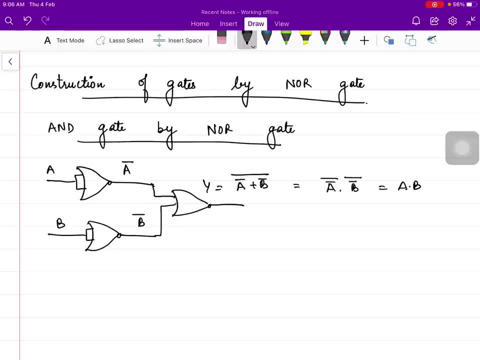 into one NAND gate. Similar. the same strategy will follow when you have to realize: AND gate by NOR gate, all right, Now, OR gate. if we see: OR gate by NOR gate, NOR gate is simply A plus B, whole bar and OR gate is simply A plus B. so you have to just remove the. 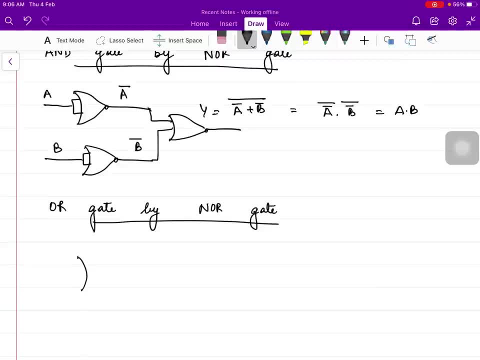 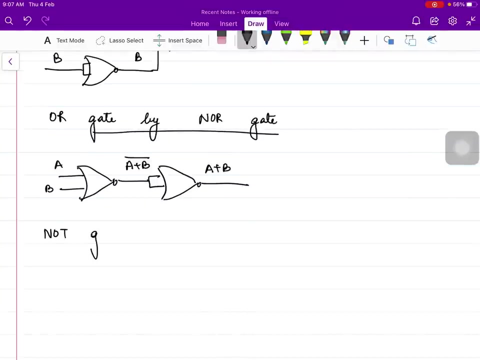 bar. So this is NOR gate A- B. it gives you A plus B bar. short the two inputs and short the two inputs, Put feed this output to this NOR gate. again you will get A plus B because this bar will be removed. so, which is very simple. Similarly, NOT gate by NOR gate. 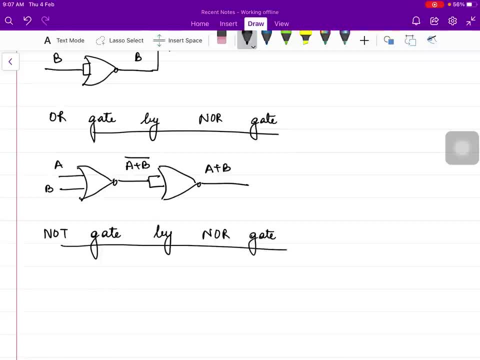 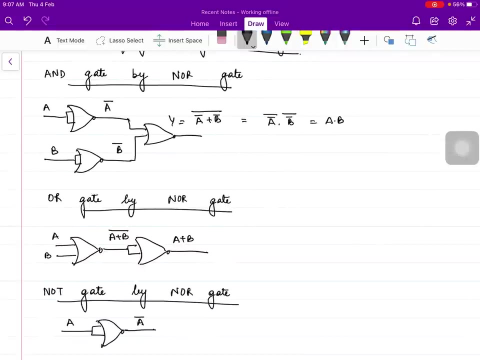